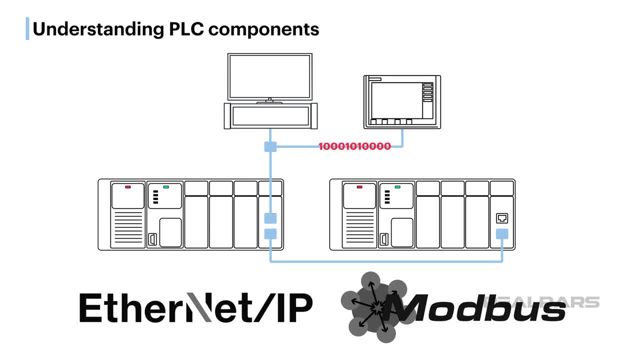 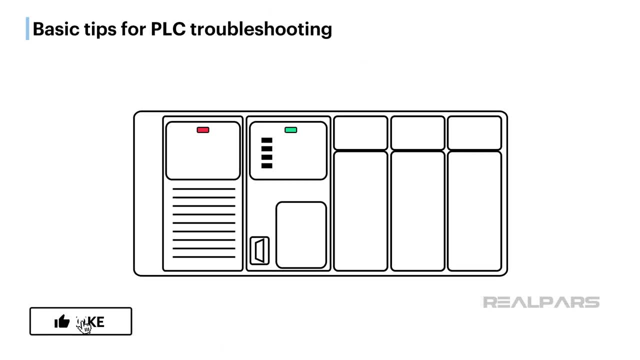 such as Ethernet, IP or Modbus to exchange data with other devices, but there are many communication protocols that exist. Now let's discuss several basic tips and steps to take during the troubleshooting process. You'll want to start by gathering as much information as possible. 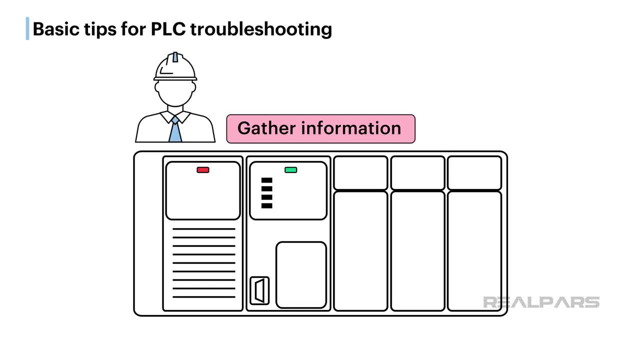 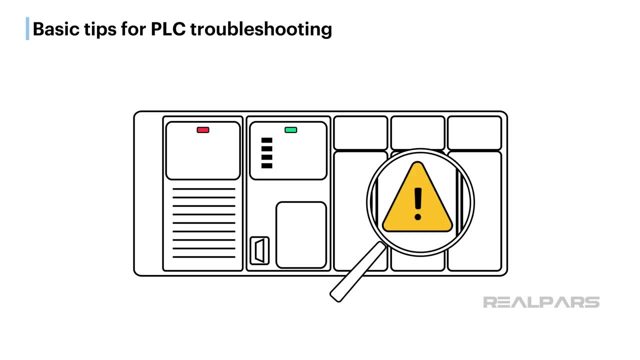 such as speaking with operators and engineers, reviewing data trends and going out to witness the issue. Pinpoint the problem by identifying a specific system or component. Troubleshoot by using trial and error methods and recording the outcome of each alteration Once a solution is proposed. 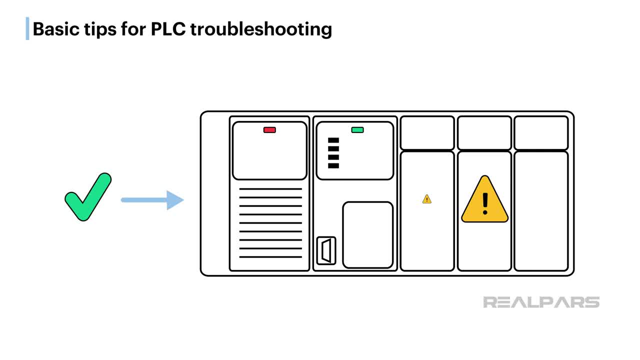 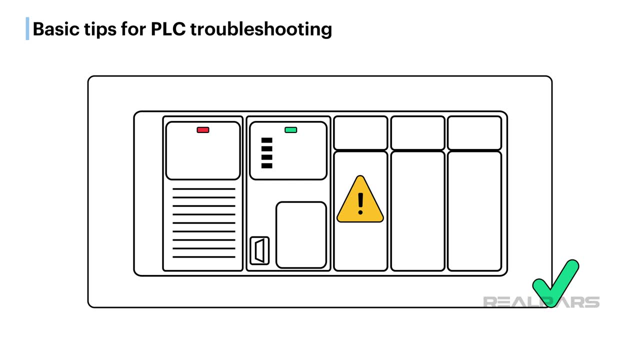 be cautious when implementing changes and consider adverse effects, Verify and test the solution. Then take careful notes and notify appropriate individuals to prevent future issues. It's important to fully understand the problem and follow a structured approach to achieve successful troubleshooting During this process, 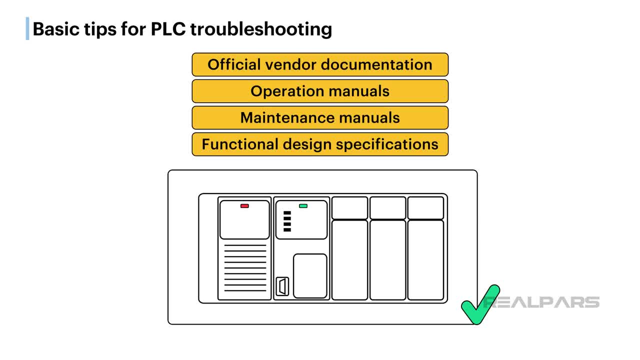 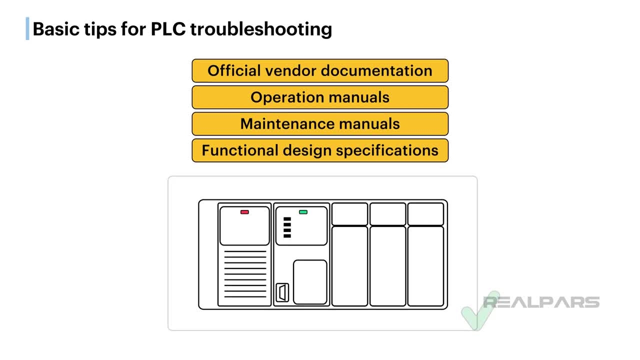 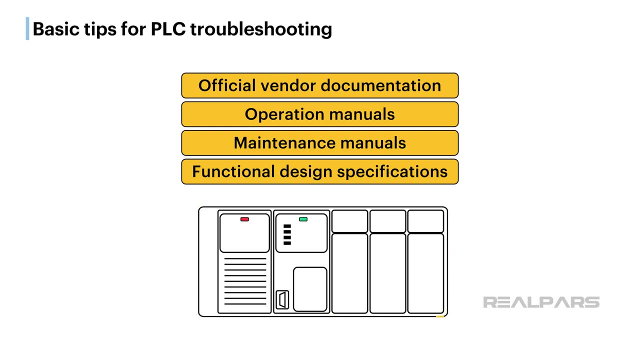 it is crucial to use resources such as official vendor documentation, operation and maintenance manuals and functional design specifications. These resources can provide valuable insight into the system and may contain troubleshooting steps specific to your PLC or control system. Don't underestimate the power of the Internet. 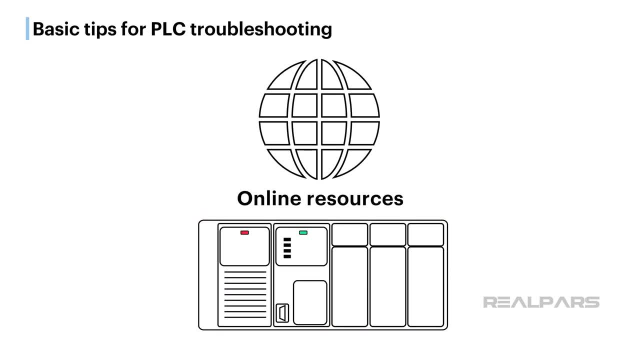 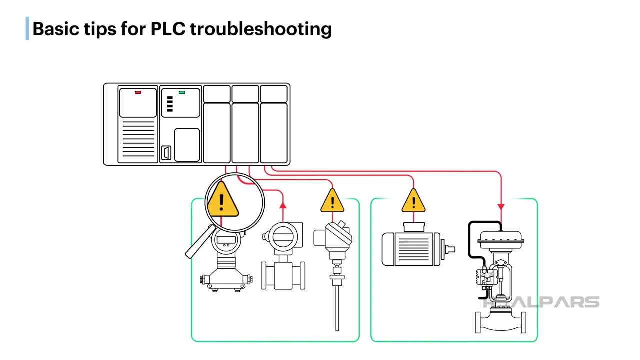 when troubleshooting your PLC. Online resources such as videos and forums can provide helpful tips and solutions from other professionals who have encountered similar issues. It is common to experience issues with wiring in a control system. You'll want to check for correct wiring throughout your PLC and control system. 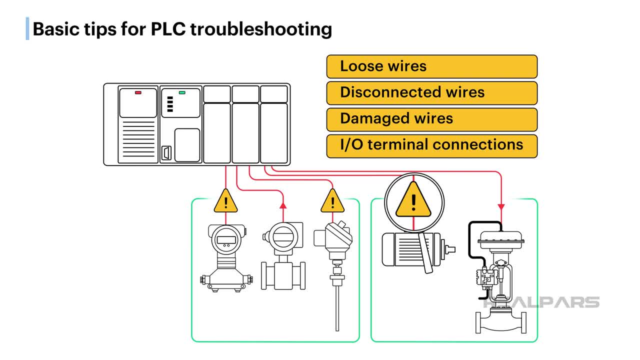 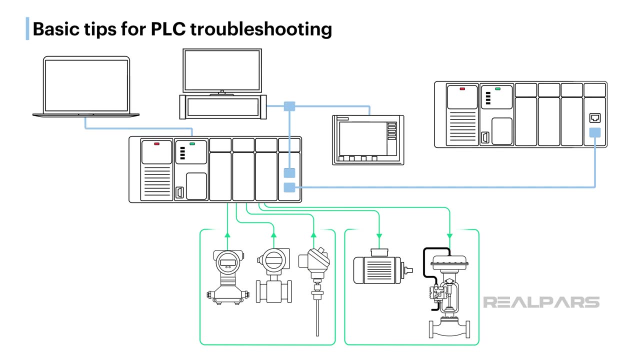 This includes checking for any loose, disconnected or damaged wires, as well as ensuring that everything is connected to the right input and output terminals. You'll also want to pay close attention to the main PLC components we touched on earlier. Verify that your power supply is working properly. 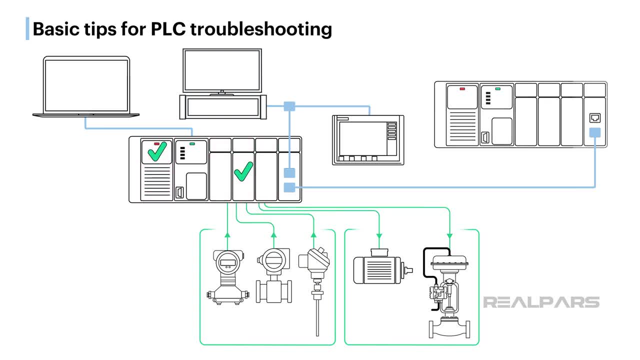 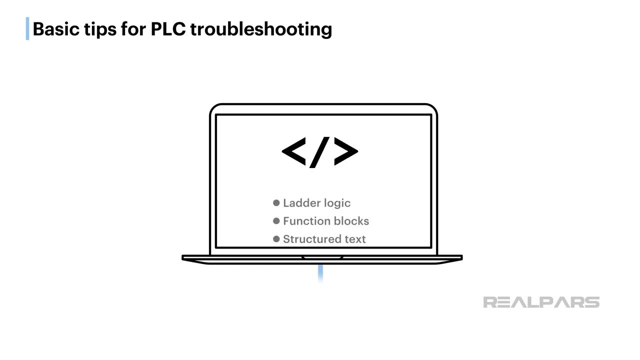 your IO modules are wired correctly and that they have been configured properly in your programming software and that all PLC communication is wired up right and configured correctly. Finally, examine the program logic. This means looking at the ladder logic function blocks. 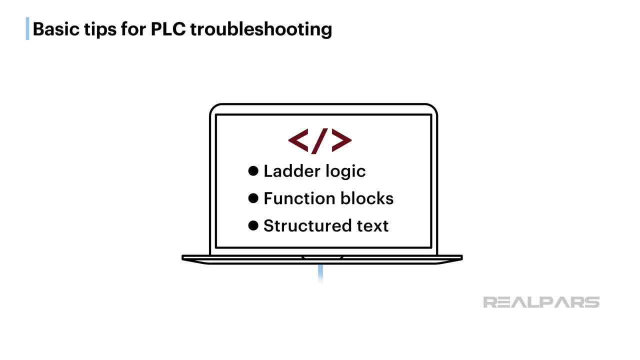 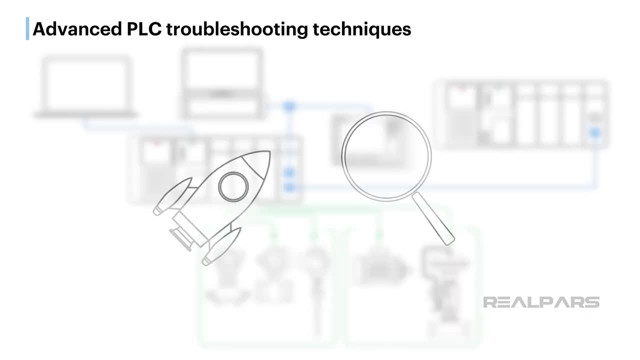 or structured text in your PLC program to see if there are any errors or issues. This can be a bit more complicated, but it's essential to identify any issues in the programming that may be causing problems. Let's touch briefly on some more advanced PLC troubleshooting techniques. 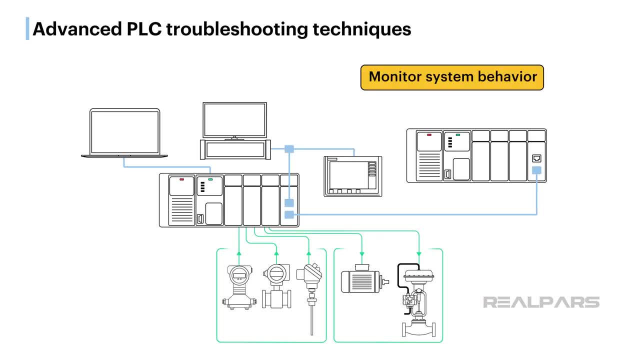 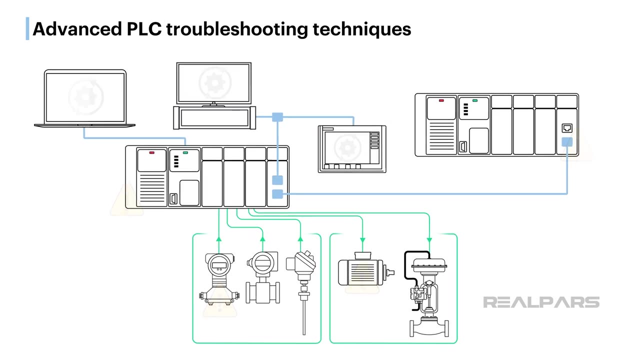 First up, let's talk about monitoring system behavior. This involves examining the system's performance and identifying any unusual behavior. This can be done through a variety of tools, such as trending alarms and event logs. By carefully monitoring the system, you can detect patterns that can reveal issues. 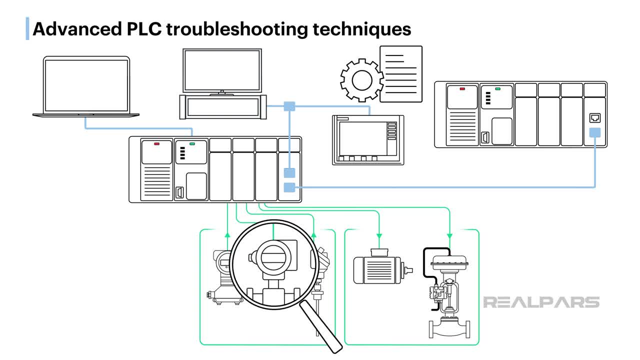 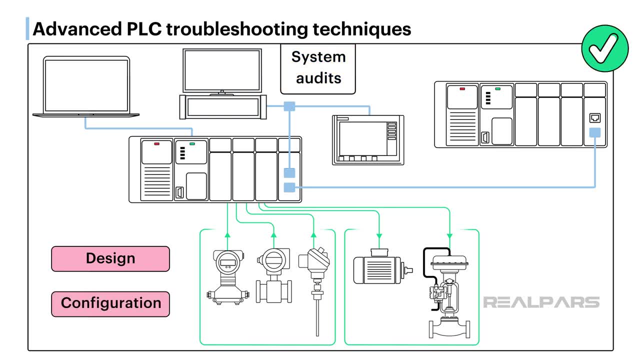 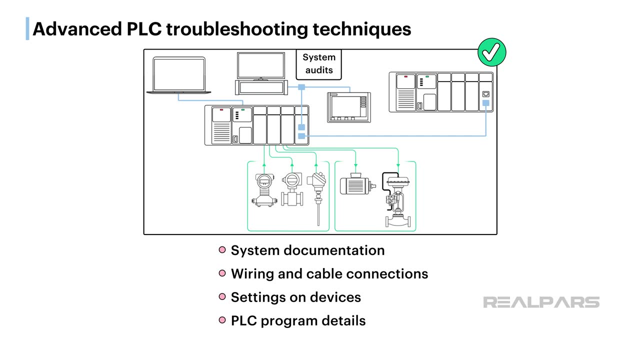 to help you toward a solution during troubleshooting. Next, we have system audits. This involves reviewing the system's design and ensuring that it is properly configured. This can be done by examining the system's documentation, checking wiring and cable connections, verifying settings on devices. 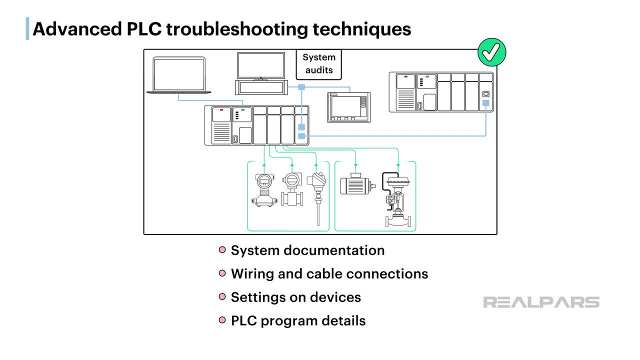 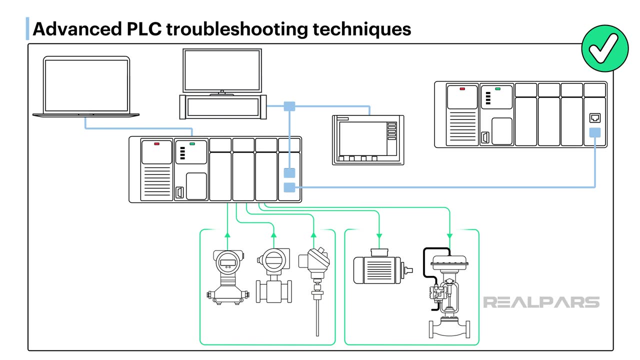 and diving into the nitty-gritty details of the PLC program. Take careful notes during system audits so that they can be compared and contrasted against similar items within your system. PID loop tuning is another technique that can be used to optimize the performance of a control system. 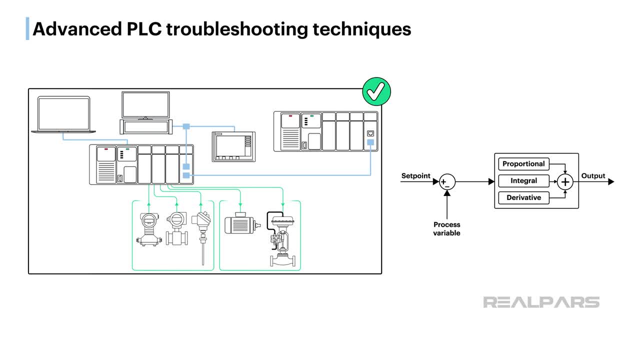 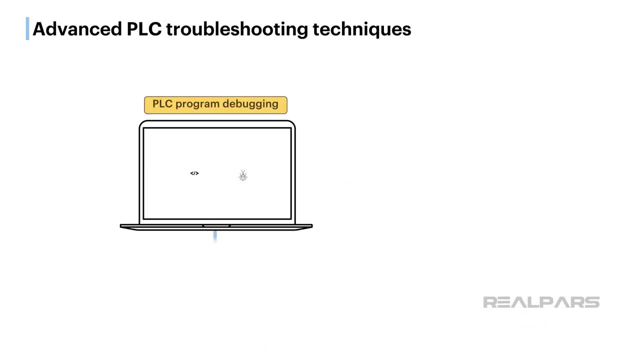 This involves fine-tuning the parameters of the PID controller to ensure that the system responds quickly and accurately to changes in the process. variable PLC program debugging is also a useful tool when working with more complicated PLC code. Program debugging is a methodical approach to problem solving. 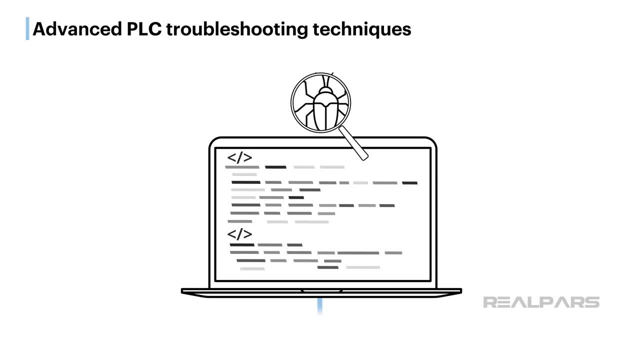 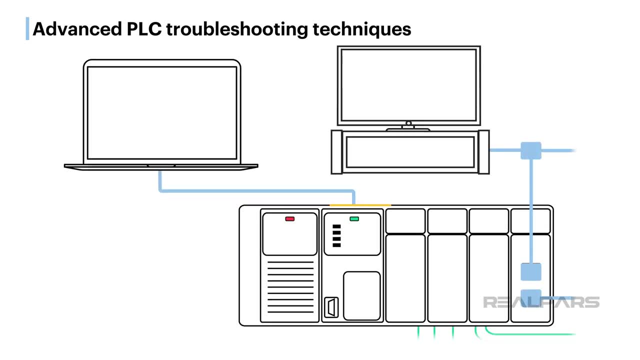 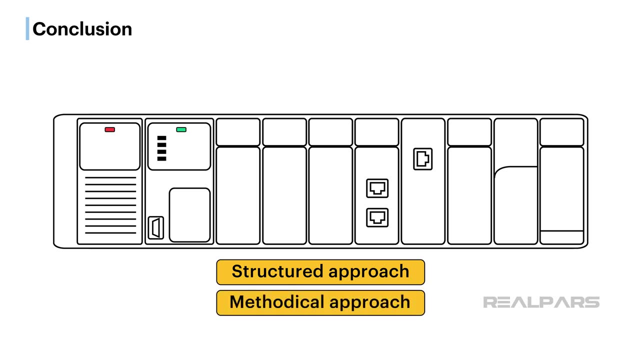 and often involves taking steps through the code to pinpoint where errors are occurring. The various debugging tools available to use will depend greatly on the PLC brand and software that you are using. PLC troubleshooting requires a structured and methodical approach, Understanding the fundamental components of a PLC. 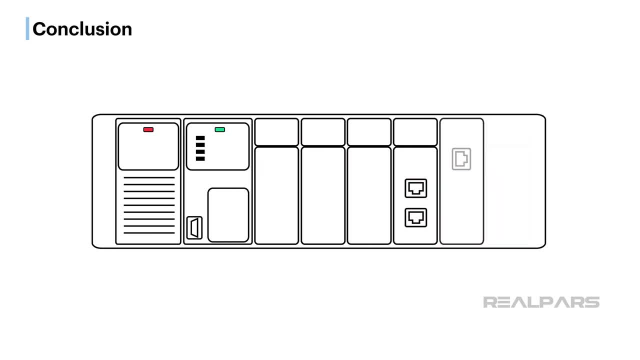 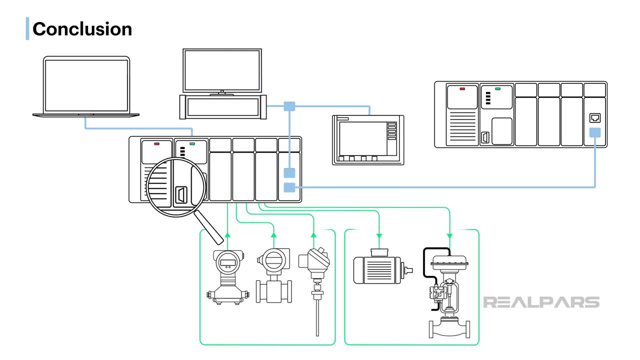 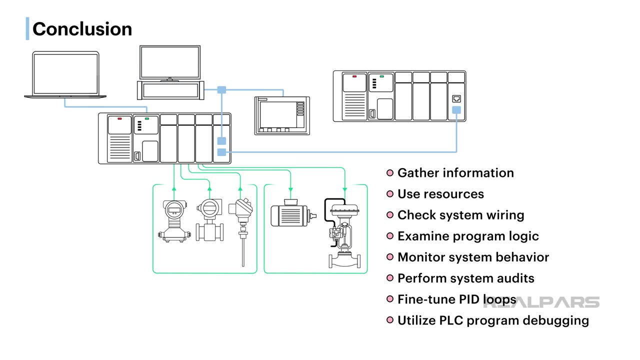 and how they work together is essential. By following basic tips and utilizing advanced techniques, you can effectively troubleshoot your control system and minimize downtime. Remember to gather information, use resources, check system wiring, examine program logic, monitor system behavior, perform system audits.